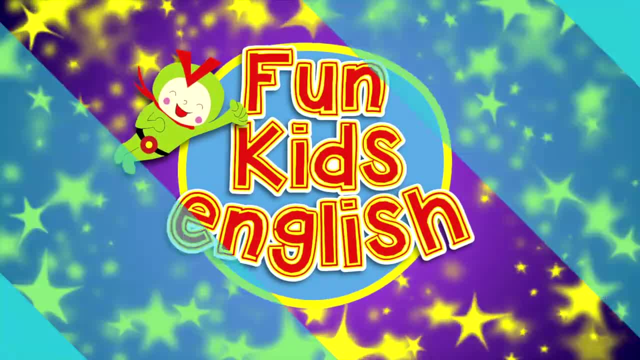 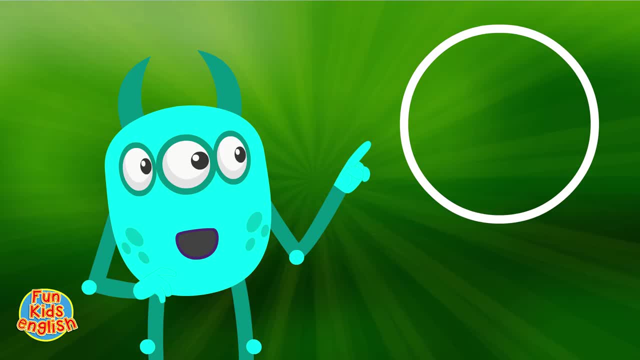 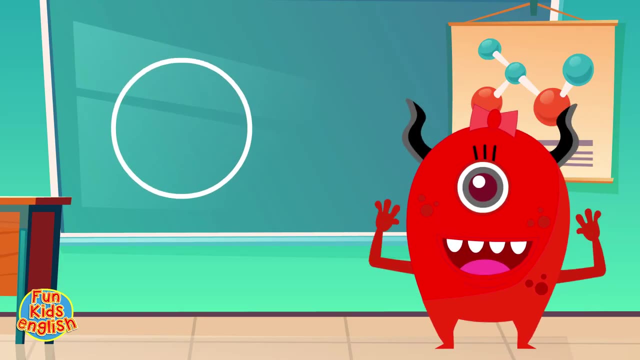 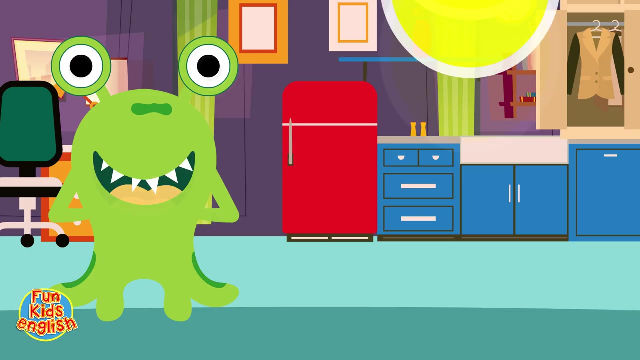 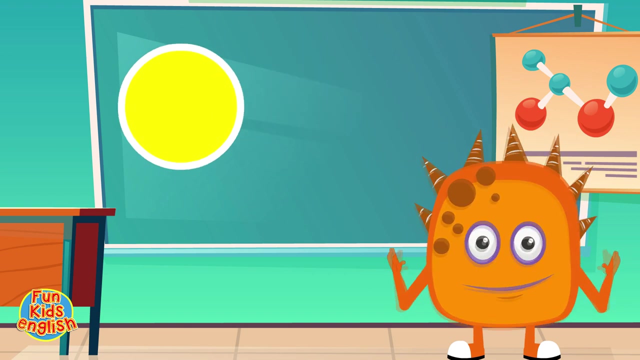 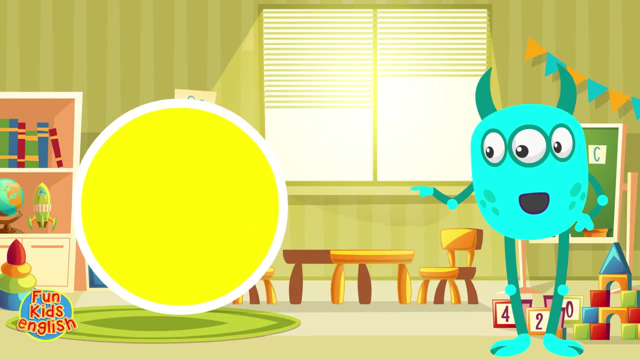 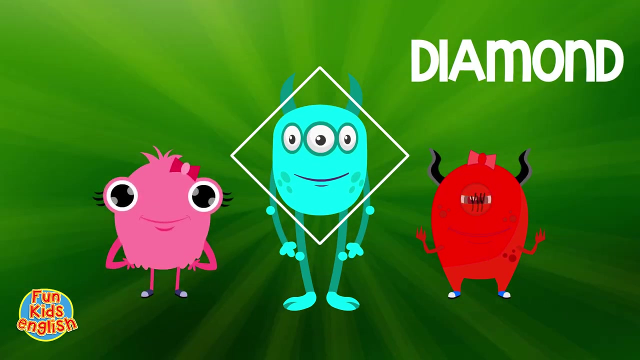 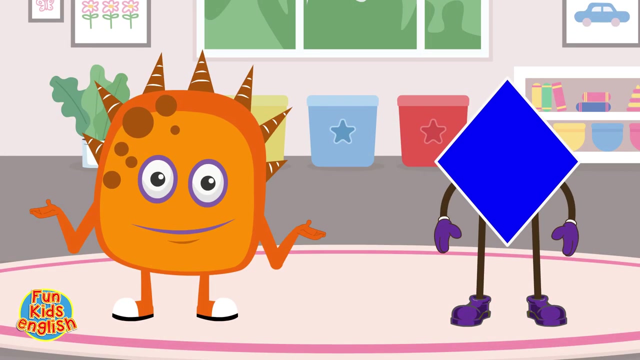 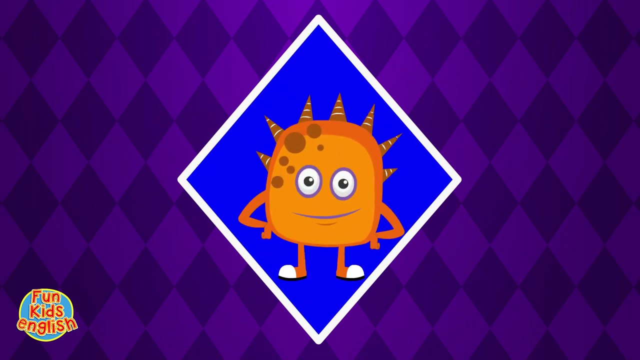 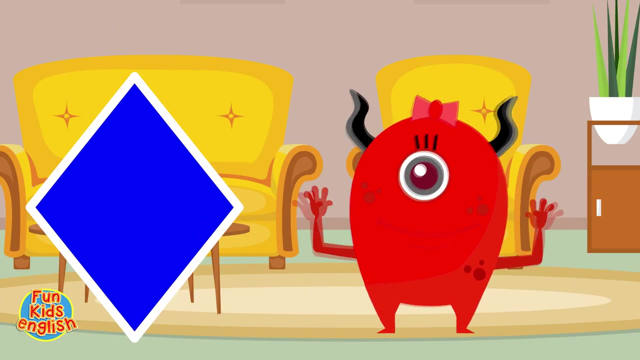 Let's make a circle. Put your hands together and make a circle. It's a circle, Yellow circle. It's a yellow circle, Yellow circle. It's a yellow circle, Yellow circle. Put your hands together and make a diamond Ready. It's a diamond, Blue diamond. It's a blue diamond, Blue diamond. It's a blue diamond, Blue diamond. 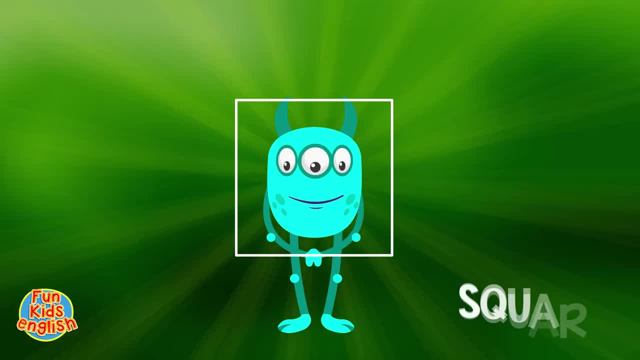 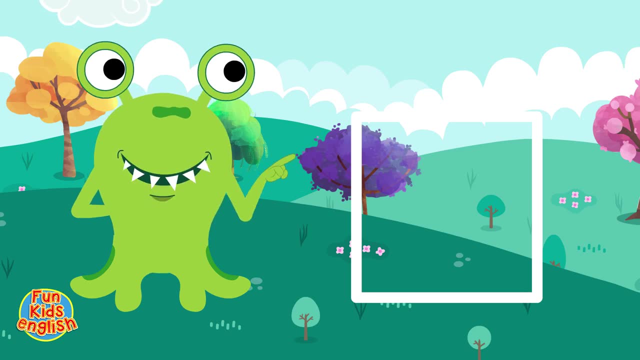 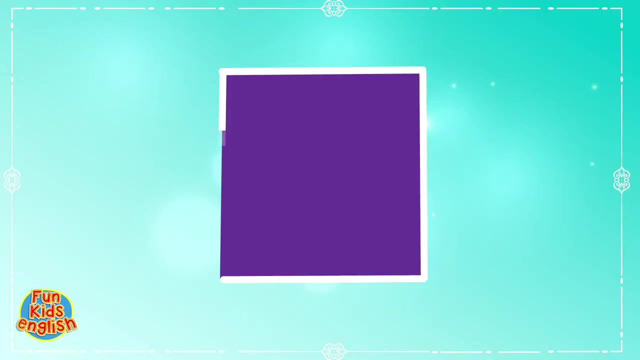 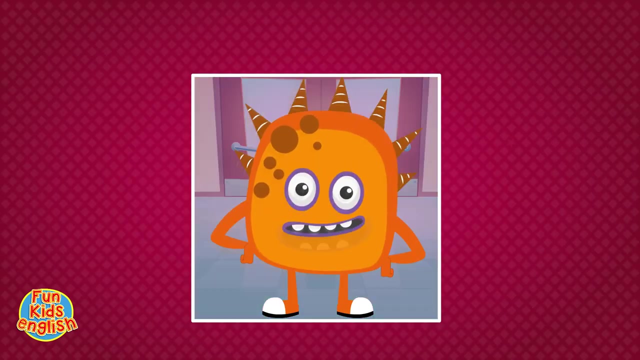 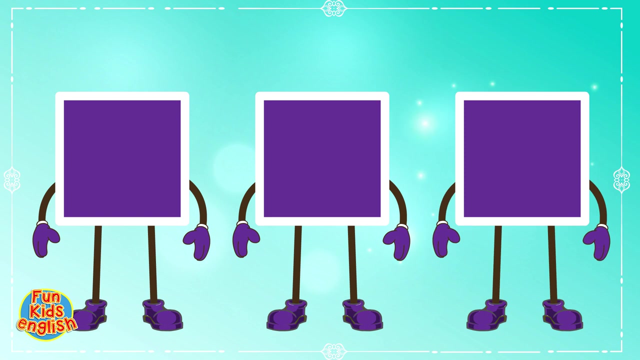 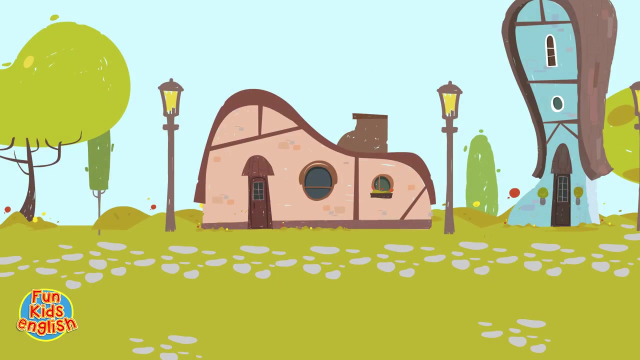 Next, put your hands together and make a square. Here we go. It's a square, Purple square. It's a purple square, Purple square. It's a purple square, Purple square. Put your hands together and make a heart. Here we go. 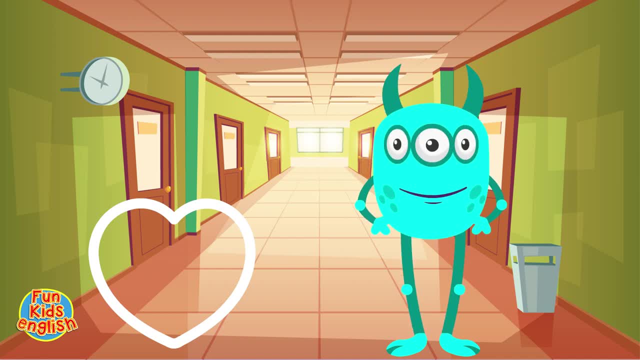 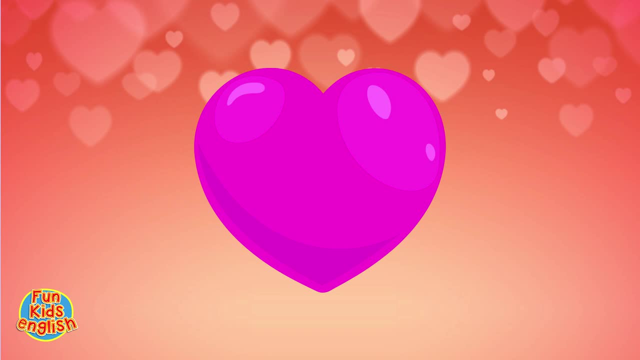 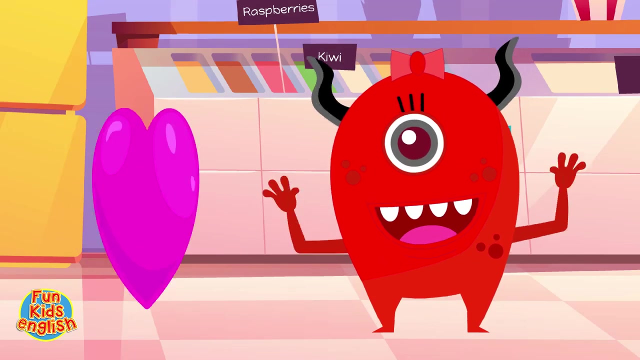 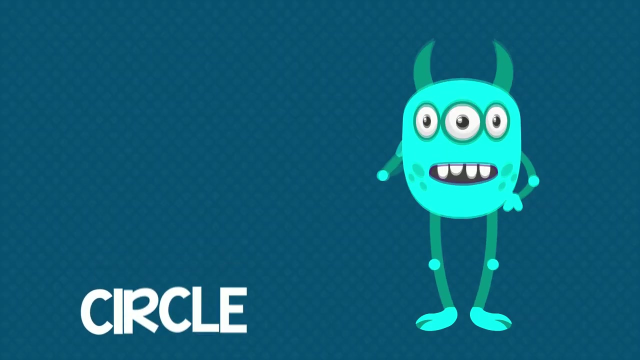 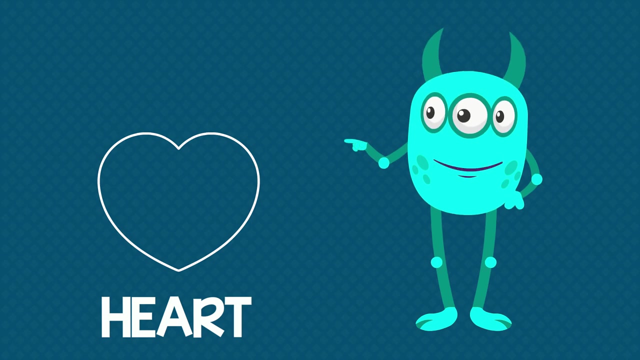 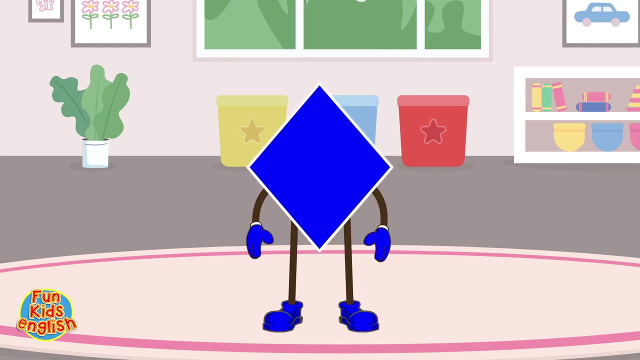 It's a heart, Pink heart, It's a pink heart, Pink heart, It's a pink heart, Pink heart. Let's make a circle, a diamond, a square and a heart: Yellow circle, Blue diamond, Purple square, Pink heart. 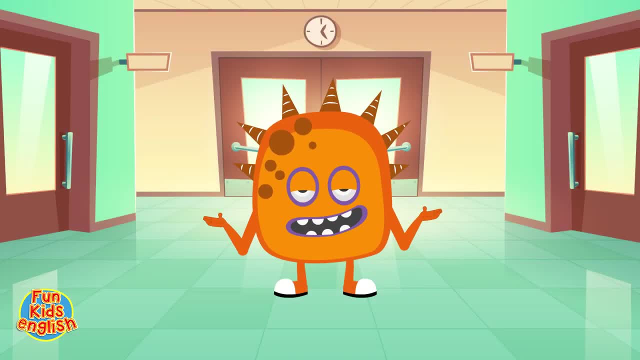 Thank you, everybody, Say goodbye, Say goodbye, Goodbye.